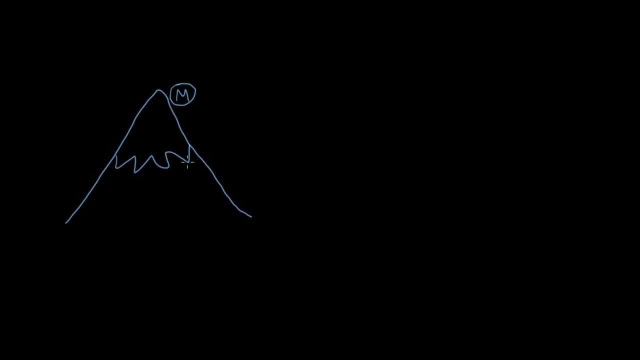 And I'm gonna put a mass here. Here's a mass of some mass m And it was lifted up to the top of the hill somehow by a ski lift, by a mountain climber, something like that. And if I put it on top of the mountain and I let it go, 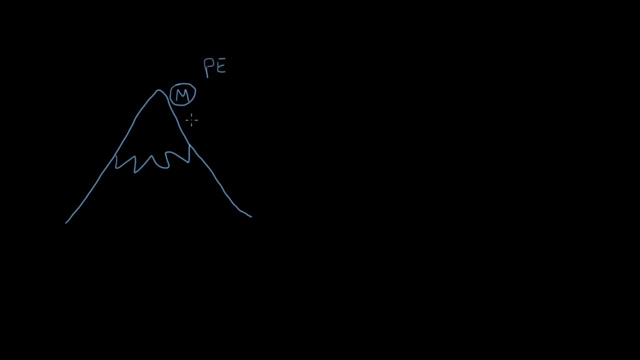 the potential energy that it has is going to be dissipated as kinetic energy And that mass is gonna roll down the hill to here And as it does, it can do some work. It can hit some trees. Let's draw a tree. 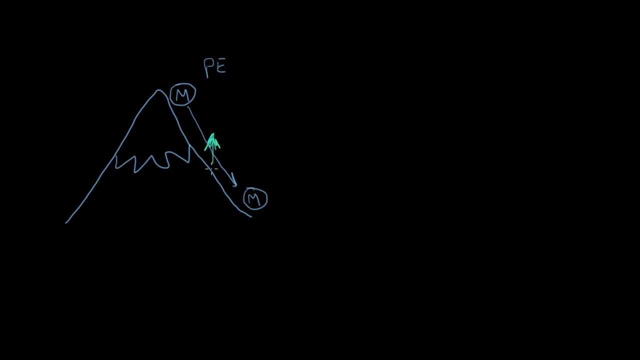 And it can run into a tree and knock that tree around, It can hit a bear, It can bounce off rocks, all kinds of things. So that's a mass rolling down a hill. Now, if I draw, this is a way to think about voltage. 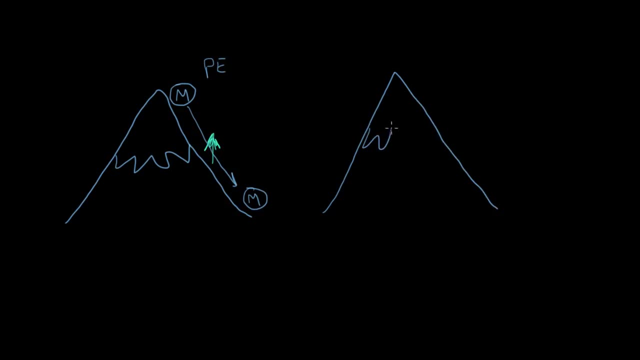 Think about voltage as being another mountaintop, And this time we'll put a battery in here. This is our battery. This is what a battery does for us: It actually builds our mountain. The battery actually delivers electrons to the top of the hill. 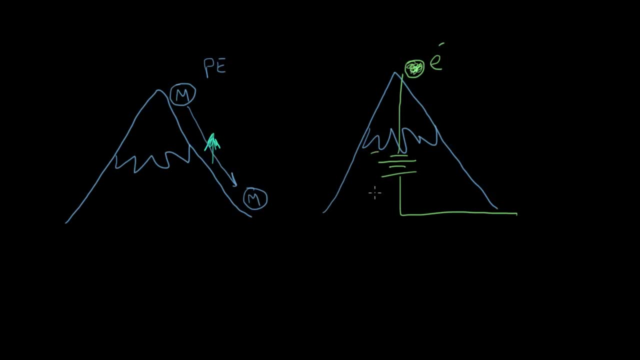 So here's an electron coming out of the battery terminal, the negative battery terminal, And if I release this, it is gonna roll down the hill And eventually it's gonna return to the bottom side of the battery, But the same thing. this is the image you have in your head. 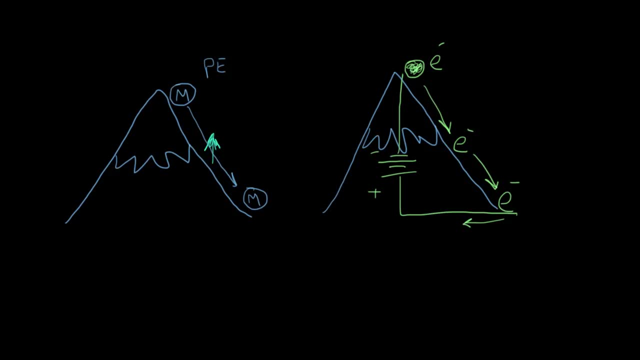 when we hook up a circuit Along the way, I can put in different circuit components like resistors or capacitors or anything like that, And I can make this electron do work and bump into things as it goes down. So the amount of voltage here is proportional. 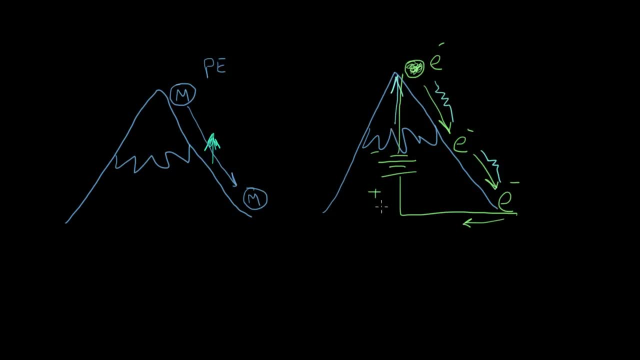 to the height of this mountain. A high voltage is a high mountain And a low voltage is a low mountain. The electrons are pushed out the top by the battery, roll down to the bottom doing work along the way, And this is where we do our circuit design. 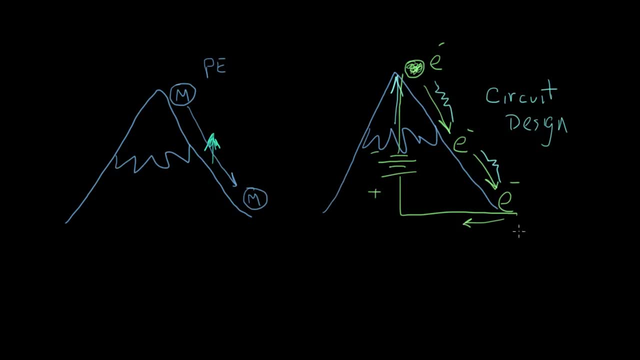 That's what we're doing over here. We buy batteries and we do our circuit design and study over here. So this is a pretty good analogy for thinking about voltage as you begin to build your circuits. See you next time.